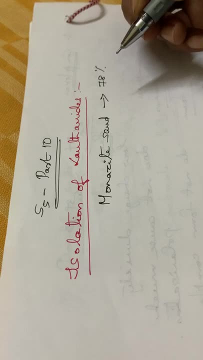 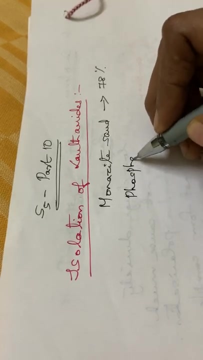 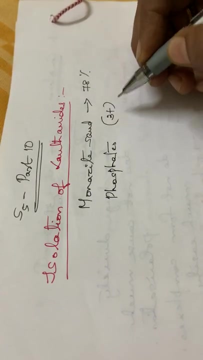 it is obtained from this monoxide sand. okay, And again these lanthanides. they are present in monoxide sand in the form of phosphates. They are present in the form of phosphates, Usually these lighter elements, or trivalent elements, that is, trivalent ions, in the form. 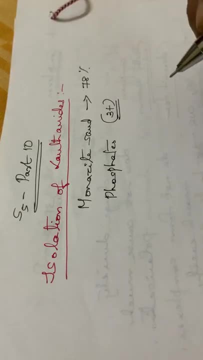 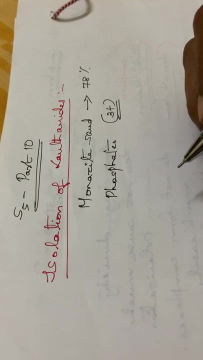 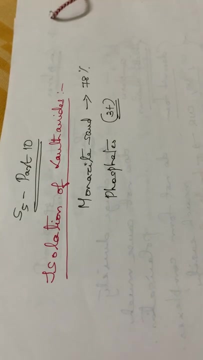 of 3+, the oxidation. with oxidation state 3+, they will be existing in the form of phosphates. Then, first of all, this is a very tedious process, and also the process, the isolation, it will be like this: The separation of lanthanides. 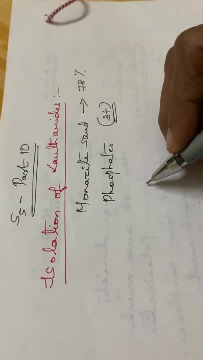 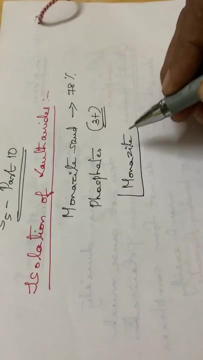 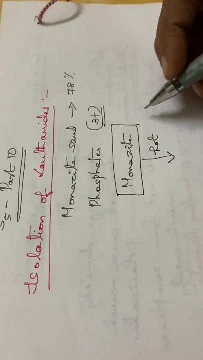 it will be like this: The first step, that is more from the monoxide sand. we are having this lanthanides in the monoxide sand. So the first step is this monoxide sand is treated with hot concentrated sulfuric acid. In your textbook it is there a flowchart, is there? 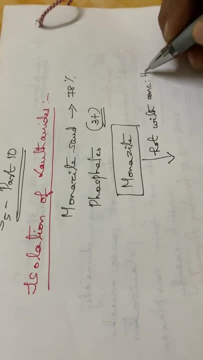 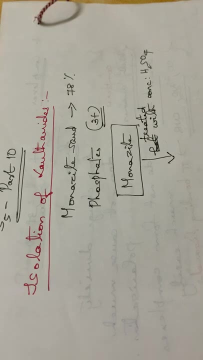 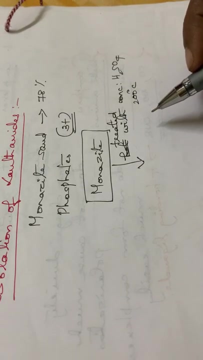 It is treated with hot concentrated sulfuric acid. Sorry, treated with hot concentrated sulfuric acid. So the temperature here it is about 200 degree Celsius. So here, while treating with concentrated sulfuric acid, it will be converting to the phosphate form, okay. So here the 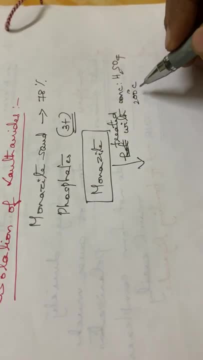 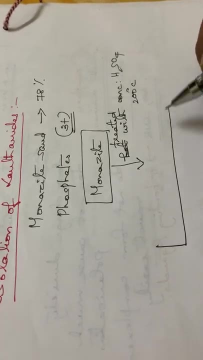 phosphates present in this monoxide sand, it will be converted to sulfates. Sorry, it is converted to sulfates while treating with sulfuric acid, so that we will be obtaining this lanthanide elements as a paste of the sulfates. That means it consists. 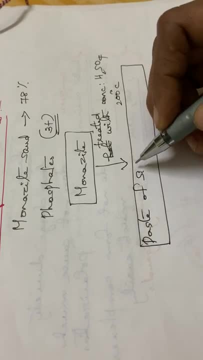 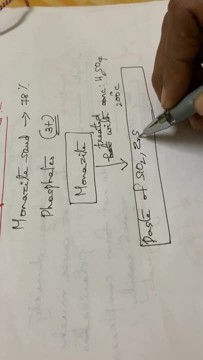 of a paste of silica. Silica, the formula is SiO2, okay, It consists of a paste of silica. then zircon. Zircon, the formula is ZrSiO4, okay. Silicone, then other sulfates of lanthanides. It. 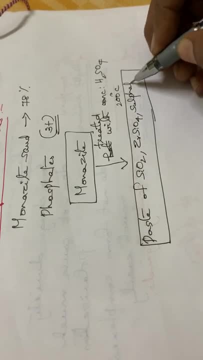 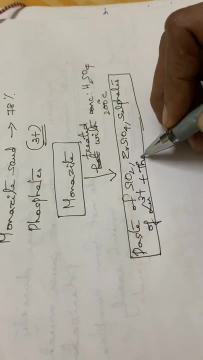 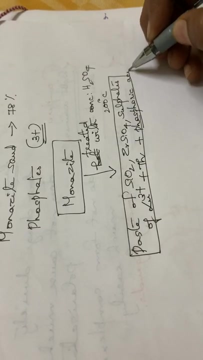 consists of silica, then zircon and other sulfates of lanthanides. okay, I am writing it as Ln3 plus, okay, And also, along with that, thorium will be present and also some phosphoric acid will be there. Phosphoric acid will be there, okay. So this is the first step: treating with concentrated sulfuric. 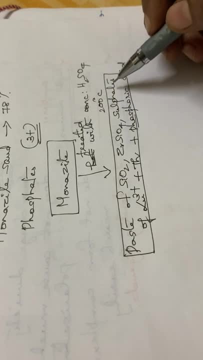 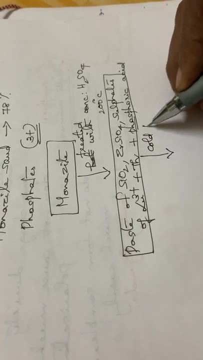 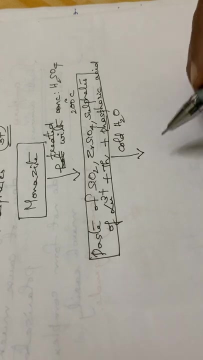 acid at 200 degree Celsius. So the phosphates will be converted to sulfates. Then in the next step, it is treated with cold water. okay, It is treated with cold water. So on treating with cold water, what happens? The sulfates will be passing into solution. So we will be having two categories. 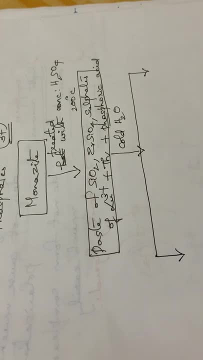 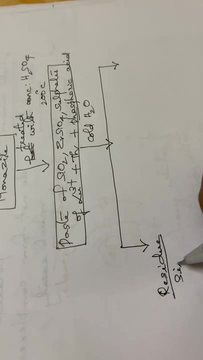 One residue we will be having and one solution we will be obtaining. And also this residue. it consists of this residue part. it consists of silica as well as zircon Silica, that is, SiO2, and then zircon- Zircon. 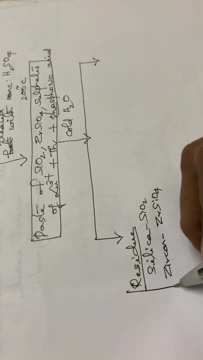 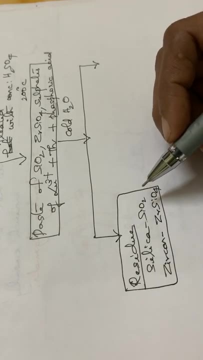 the formula is ZrSiO4,. okay, The residue part. it will be having silica and zircon that we can separate. That means it remains undissolved. You know the form of precipitates, is not it? So here also it will be remaining as solid and we can separate this part. 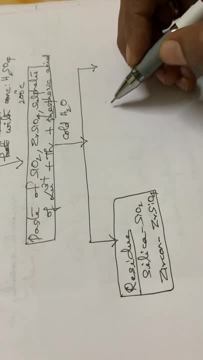 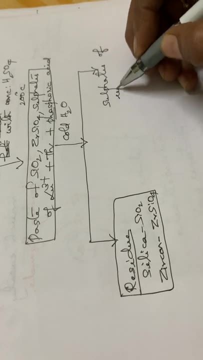 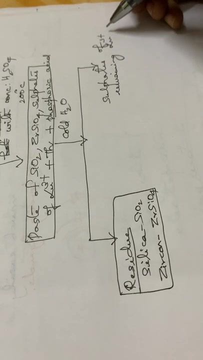 zircon. we can separate. Then the next part in the solution. we will be having the sulfates of remaining lanthanides. Sulfates of remaining lanthanides- okay, Sulfates of remaining lanthanides plus thorium plus. 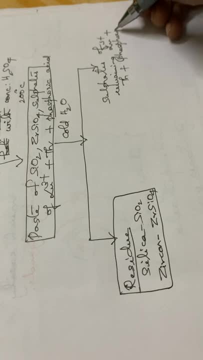 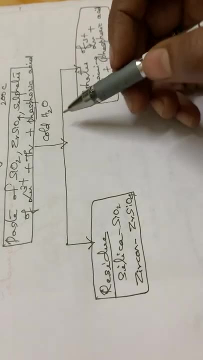 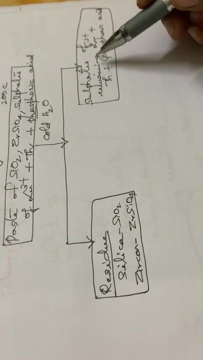 phosphoric acid. This will remain in the solution. So from the solution we have to isolate the other lanthanides also. okay, So this: while treating with cold water, we will be having a residue and a solution. The residue will be having silica as well as zircon And in the solution 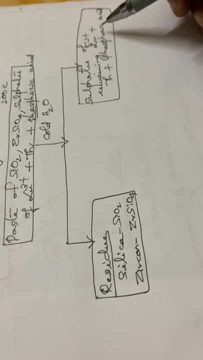 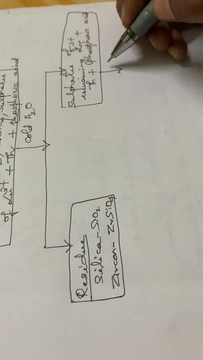 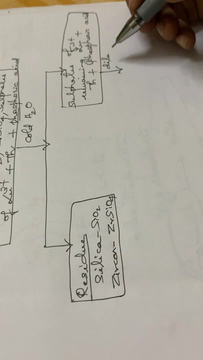 we will be having sulfates of lanthanides, then thorium and phosphoric acid. Then in the next step we have to isolate this thorium. okay, So for isolating this thorium we have to dilute this solution, or we have to add water to the solution And again this: it is then diluted. 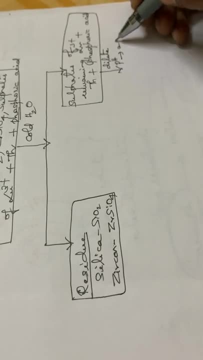 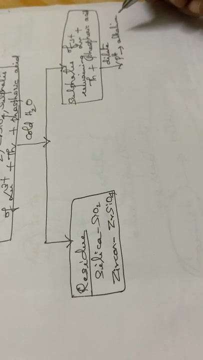 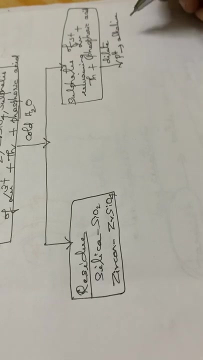 Then it is the pH range. it is adjusted to alkaline medium. okay, The pH range is adjusted to an alkaline range. So what happens is that the sulfates pass into solution. it will be remaining in the solution And also while adjusting this pH, what happens is that 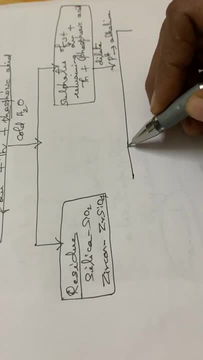 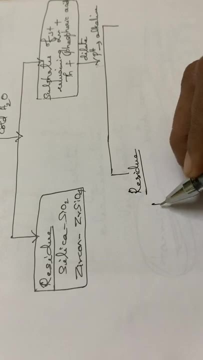 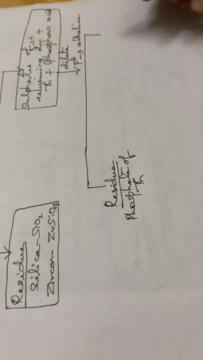 we will be having again two categories. That means one residue and one solution. okay, This received. we will be having the phosphate of thorium. okay, in the residue we have phosphate of thorium, so that thorium is isolated. okay, and again in the next step. see here that here we will be having 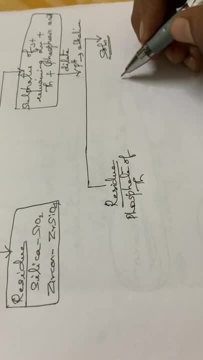 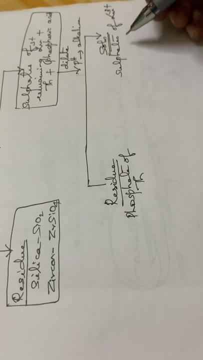 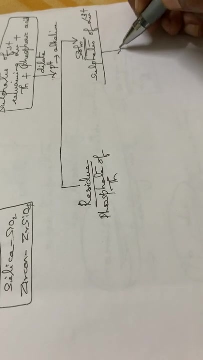 a solution, isn't it residue and the solution part, and in the solution it will be having the sulfates of lanthanates solution. it will be having the remaining lanthanates in the form of sulfate. okay, then, in the next step we have to to this solution we are adding sodium sulfate, Na2SO4. 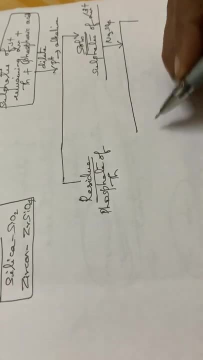 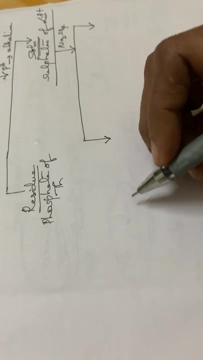 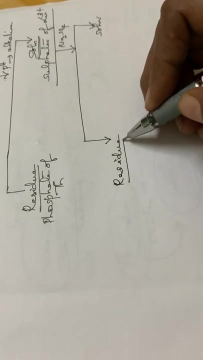 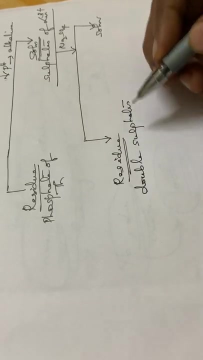 to the solution, adding sodium sulfate, so that again we will be having two categories, that is, one of them will be converted to double sulfates. that is again residue and again here we will be having solution. okay, in the residue we will be having double sulfates, double sulfates and this double sulfates, double sulfates of light, lighter lanthanates will be. 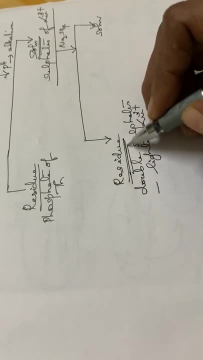 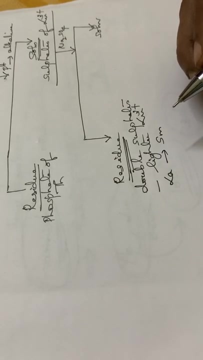 there. double sulfates of lighter lanthanates will be there present in the residue. that is from lindanum to samarium. that is the starting elements. okay, from lindanum to samarium. that is lindanum, cerium, promethium, neodymium- sorry, prasodymium, neodymium, promethium and samarium. 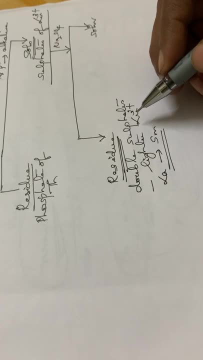 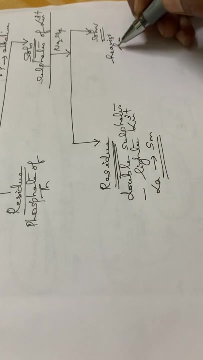 these elements will be added to the solution. okay, and again we will be having the remaining lanthanates obtained, as in the residue part. okay, and also in the solution part we will be having the heavier lanthanates. heavier lanthanates will remain in solution ln 3 plus okay, heavier lanthanates. 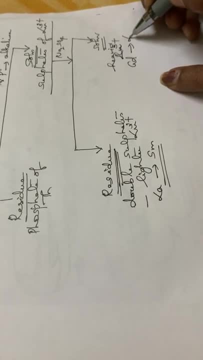 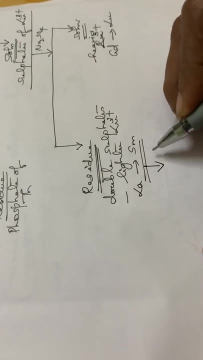 will remain in the solution that is starting from gadolinium to lutetium. the remaining lanthanates will be there in the solution. again this lighter lanthanates. again it is treated with NaOH: lighter lanthanates. when treated with NaOH, it will be having the same solution. okay and again. 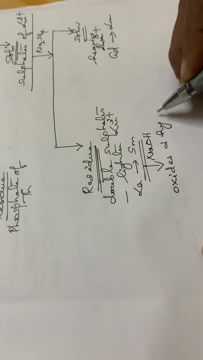 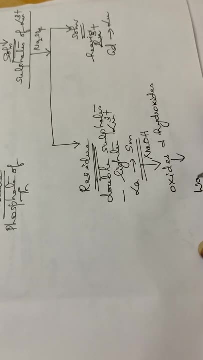 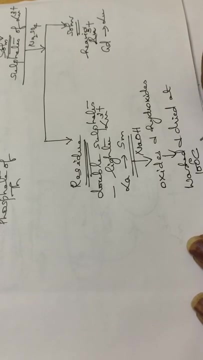 it will be converting to oxides as well as hydroxides. converting to oxides and hydroxides, then this oxides and hydroxides, then washed and dried, washed and dried at 100 degree Celsius. washed and dried at 100 degree Celsius, then we can separate by these lighter lanthanates. 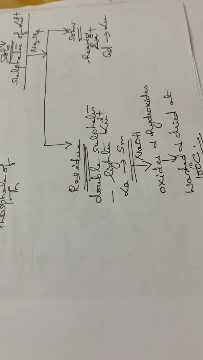 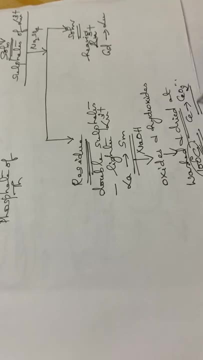 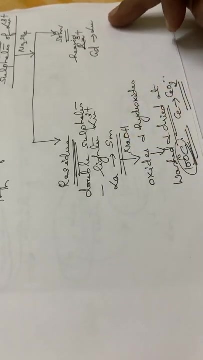 by certain different methods. okay, so here at this stage, what happens when, washed and dried at 100 degree Celsius, Serium will be oxidized to CaO2. okay, so this is the process of separation of lanthanates. so here we are, separating this lighter lanthanates as well as the heavier lanthanates, then again, 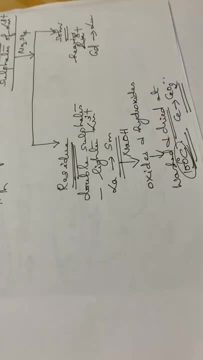 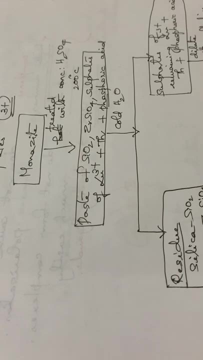 we have to follow some other procedure for separating these two categories, that is, lighter as well as heavier lanthanates. so this is the flowchart of this separation of or isolation of lanthanates. so in your textbook it is given very clearly the flowchart, so you have to. 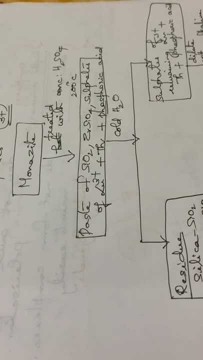 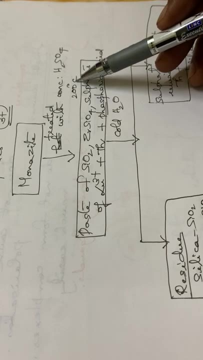 study the flowchart, Then you can write the procedure itself. for a four more question, okay, I will tell you once again this monosite sand. first, it is treated with concentrated sulfuric acid at 200 degree Celsius, so the in the monosite, this lanthanates, will be present in the form. 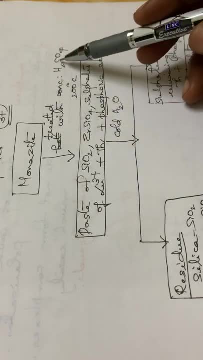 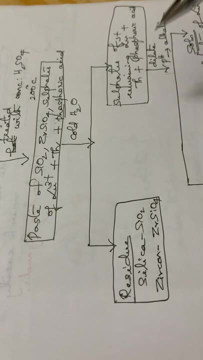 will be there in the form of phosphates. so here, treating with concentrated sulfuric acid, we will be having the sulfates. phosphates are converted to sulfates along with some phosphoric acid. then you have to dilute or treat it with cold water. then we will be having 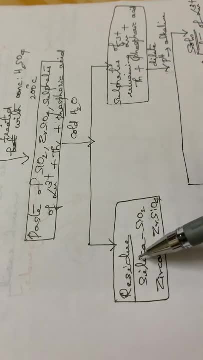 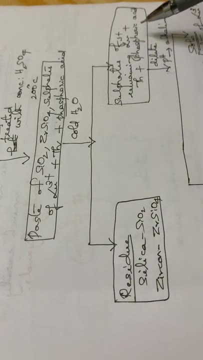 two categories. We will be having the residue as well as the solution. in the residue we will be having silica and zircon that we can separate out. that means it will be in the solid form, then in the solution the remaining lanthanates and thorium in the form of sulfates. then you 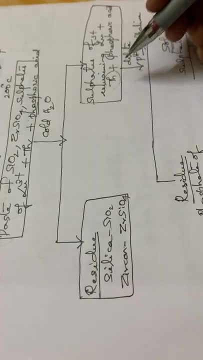 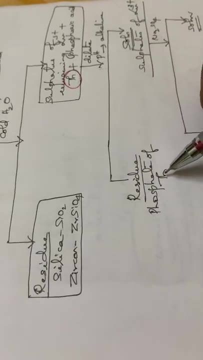 have to separate this thorium. for separating this thorium we have to adjust the pH. that means the pH will be adjusted to the alkaline range so that this thorium will be left as residue in the form of phosphate. Then again in the solution, this sulfates of phosphates will be in the form of phosphates. 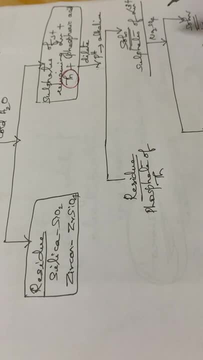 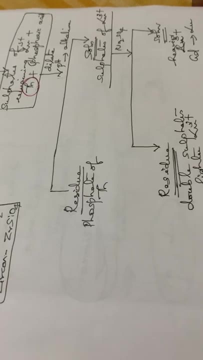 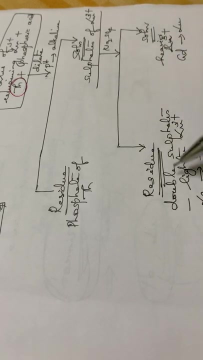 So this is the solution. Sulfate of lanthanum will be there and again it is treated with sodium sulfate. so hope you are clear. And while treating with sodium sulfate, again, we will be having two parts: that is, the residue as well as the solution, that is the lighter. lanthanates will be precipitated as a dude. 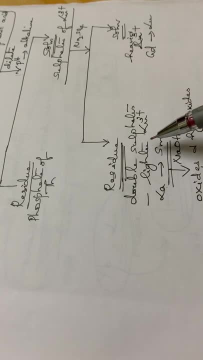 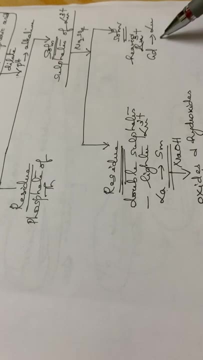 sulfates. that is starting from lanthanum to samarium. we will be. We will be having the light lanthanates and they will be precipitating their and the remaining lanternates, that is, the heavier lanthanate lanthanates. it will be there in the solution. then you have to do some more steps to separate each. 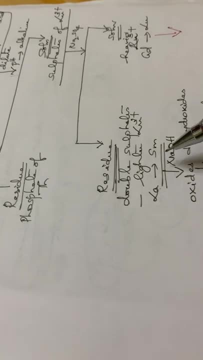 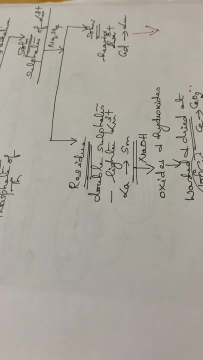 and every element from this solution. okay, and again this: this lighter lanthanates. it is then treated with naoh and is converted to. so, while treating with naoh, it is converted to oxides as well as their hydroxides. then it is washed and dried at 100 degree celsius. so while drying to, 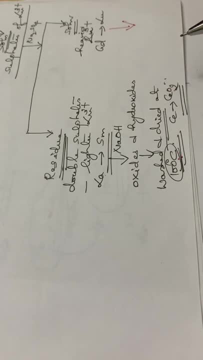 100 degree cerium, it is oxidized to ceo2. so this much is there regarding the isolation of lanthanates. okay, so you are getting a residue of the lighter lanthanates as well as a solution of a heavier lanthanates. then you have to continue with the separation of lanthanates. that means lanthanates. 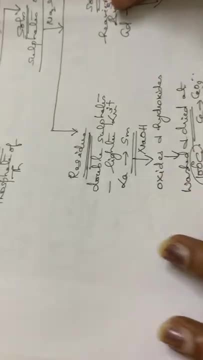 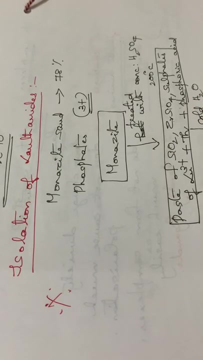 can be separated by so many different techniques and those techniques you have to study. so this isolation of lanthanates. it is very important. usually it is an asked question from lanthanate, lanthanate part. the important questions are: the first one is lanthanate contraction, then the 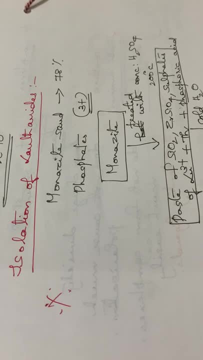 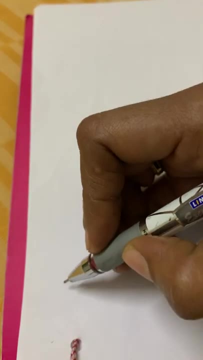 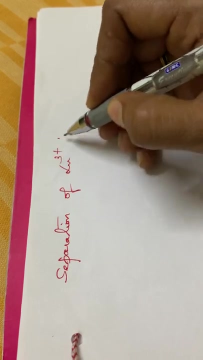 isolation of lanthanates, then the separation of lanthanates and then the separation of lanthanates of lanthanides. These are very, very important. Then the next is separation of lanthanides, Separation of lanthanides. So the first step for separation, that is the fractional crystallization. 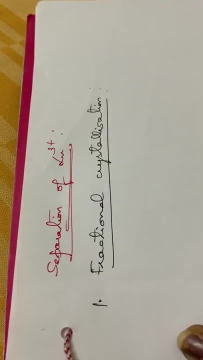 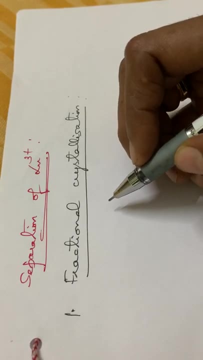 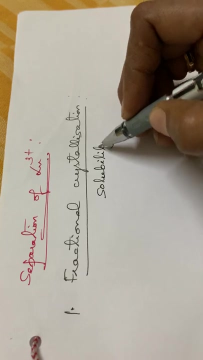 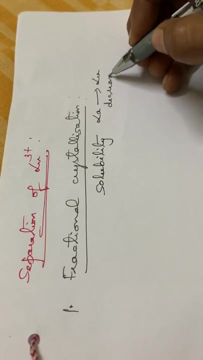 So here this fractional crystallization, the principle which is following: in this fractional crystallization, it is the solubility. We have to consider the solubility of the salts. That means the solubility decreases from lanthanum to lutetium, isn't it? Solubility decreases from 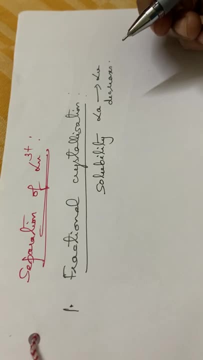 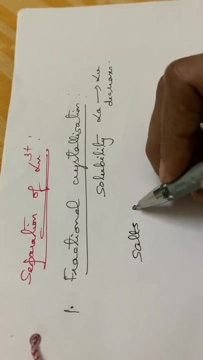 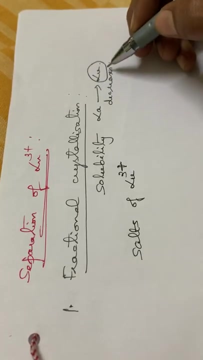 lanthanum to lutetium. So, based on this difference in the solubility, this fractional crystallization technique is adopted. That means the salts of lutetium. salts of lutetium, that means it will be coming at the end of the series, isn't it At the end of the series, this lutetium ion and also? 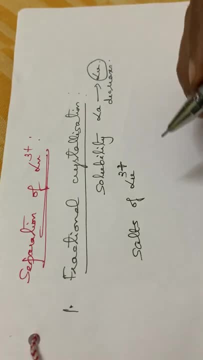 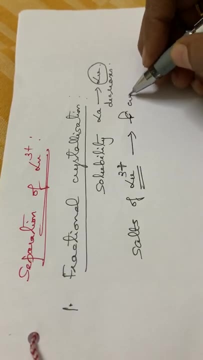 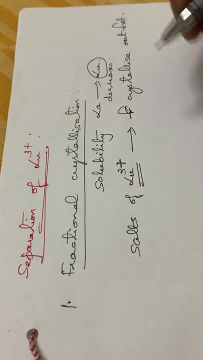 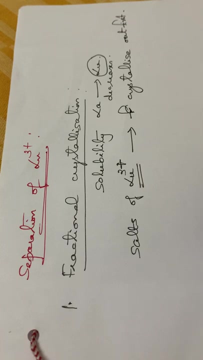 their size is also very, very low, isn't it? So what happens is that the salt of lutetium will be crystallizing out first, So lutetium salt will crystallize, will crystallize out first. Then, in the case of simple salts also, the simple salts and double salts are also this. 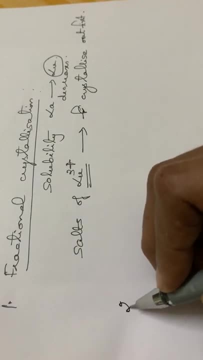 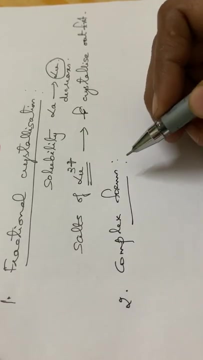 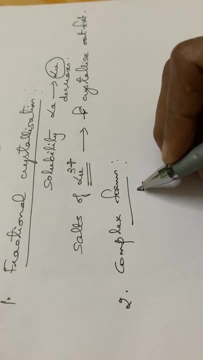 method, this fractional crystallization technique, is adopted. Then the second one, that is, the complex formation. Complex formation- See here, in the case of this, lanthanides. usually it can form complexes. Normally we are using EDTA. What is EDTA? It is ethylethionate. 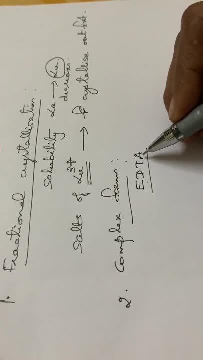 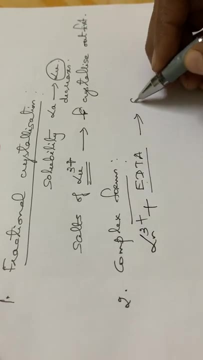 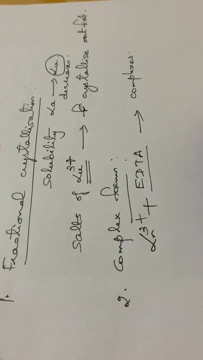 Ethylene diamine tetraacetic acid- EDTA. So usually, when treated with EDTA, this forms complexes, Lanthanides. when treated with EDTA, it forms complexes. Okay, EDTA means ethylenediamine tetraacetic acid. So what happens is that at the end of the series lutetium 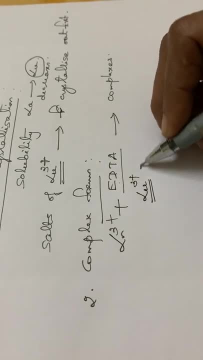 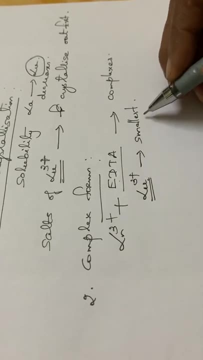 is coming, isn't it? LU will be coming, and also the ion. it is the smallest ion: lutetium 3+. it is the smallest ion. And so, since it is the smallest ion, what about the complex formed? Is it a stronger? 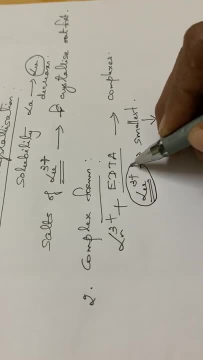 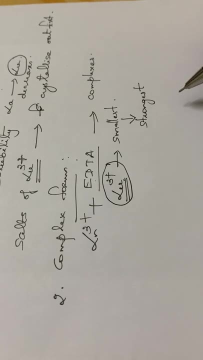 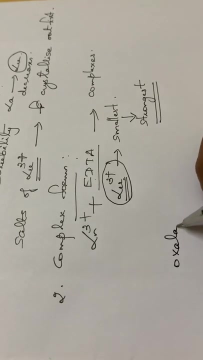 complex or a weaker complex. It is the smallest ion, isn't it? That means it can form a strongest complex. Okay, This lutetium can form the strongest complex, and also, so that is one point. Then again this: usually they can be converted into the oxalate forms, These lanthanides, 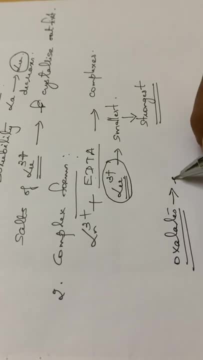 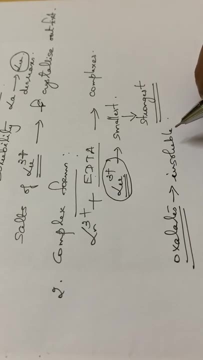 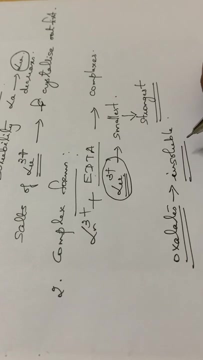 they can be in the oxalate forms, and also these oxalates. as you know, they are normally soluble in water, isn't it? Oxalates are insoluble. and also, while complexing with EDTA, these oxalate ions does not give a precipitate. Okay, And again, when acid is added to this. 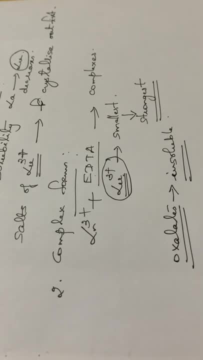 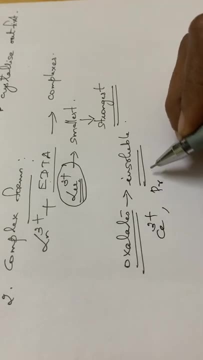 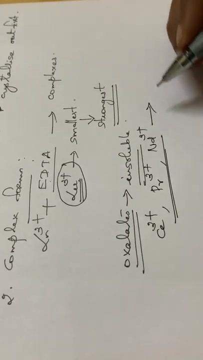 solution. the least stable complexes will be coming first or will be dissociated first. That means cerium 3+, then presodium 3+, then neodymium 3+, ND3+. These complexes, they will be forming complexes and they comes out first. Okay, That means they are precipitated as. 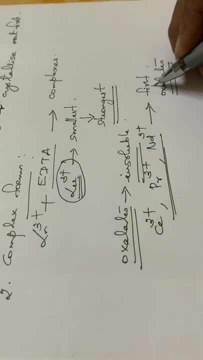 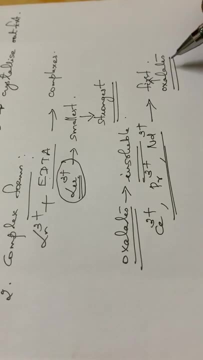 their oxalate. they are precipitated as their oxalates first, Okay, So that we can separate these complexes. and then they are filtered off and we can separate these three from the solution. Okay. And this process we have to continue so many times. So here at first. 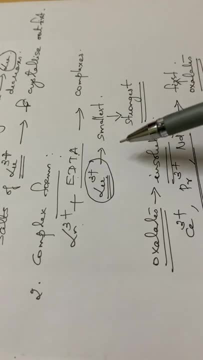 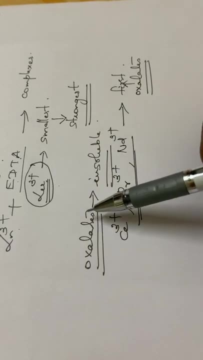 this lanthanum ions. it is complexed with EDTA, So while forming complexes, the smallest ion will form the strongest complex. Usually they are. these oxalates are. their lanthanates will be taken in the form of oxalates. 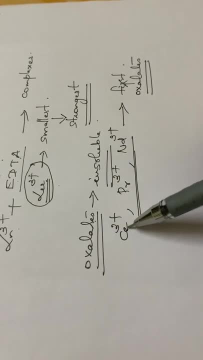 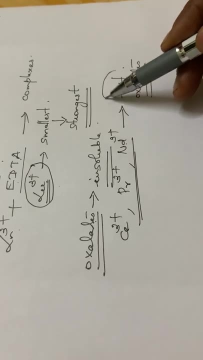 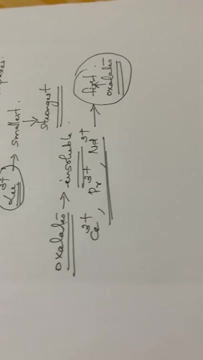 and then they are also insoluble in water. So in that case the cerium presodium, neodymium, etc. will be forming strongest, will be forming complexes, and they will be first. we can precipitate out these complexes first. Okay, Then again the next method, that is the 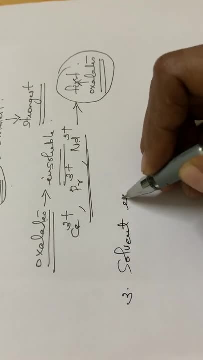 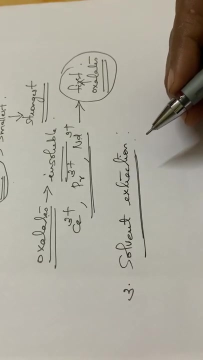 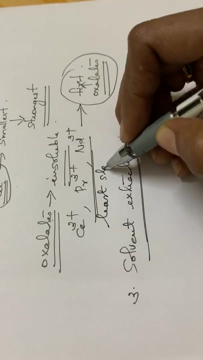 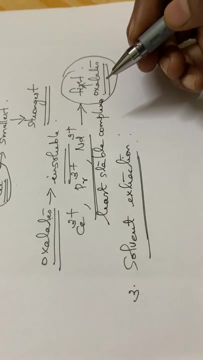 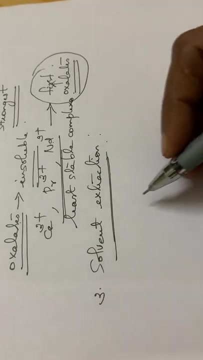 solvent extraction, Solvent extraction. Okay, Here, one more point is that these, these are the least stable complexes, isn't it? Cerium, promethium, neodymium? these are the least complexes, least stable complexes. Then the next one, that is, the solvent extraction. So here in solvent extraction. 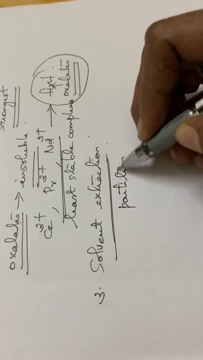 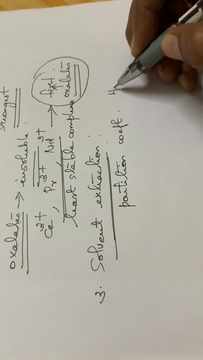 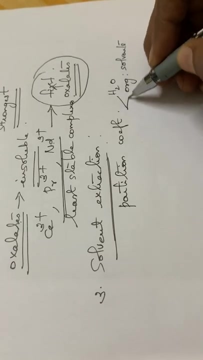 we are using the principle Partition coefficient- solvent extraction, partition coefficient of the- this lanthanate salts- between water as well as the organic solvents. Usually partition coefficients are done in in solvents, isn't it So here? partition coefficients of water as well as organic. 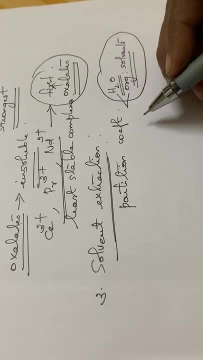 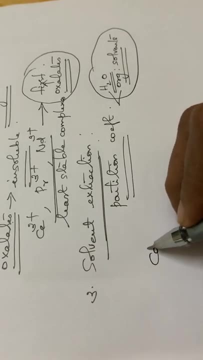 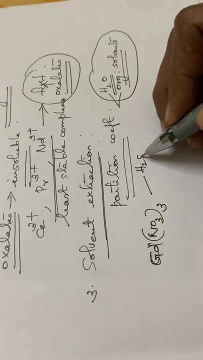 solvents here, while using this lanthanate salts. this partition coefficients are slightly different. That principle is adopted here And again. this partition coefficient of gadolinium nitrate- GdNO3- thrice gadolinium nitrate in water, as well as in n-butyl alcohol. The partition coefficient: 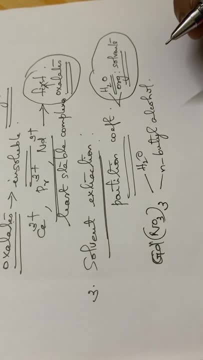 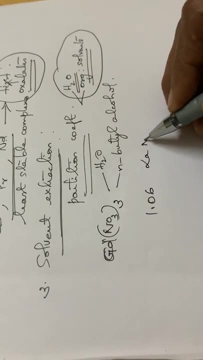 of gadolinium nitrate in water, as well as between water and n-butyl alcohol. It is it is about 1.06 times greater than that of lanthanum nitrate, LaNO3- thrice in water, as well as n-butyl. 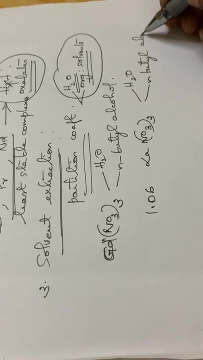 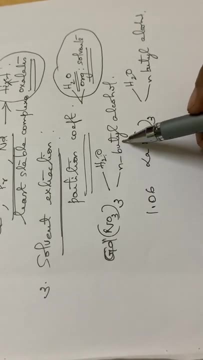 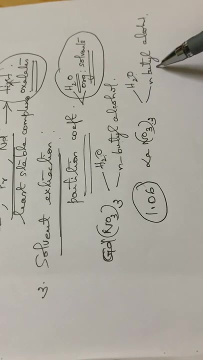 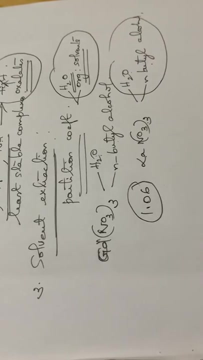 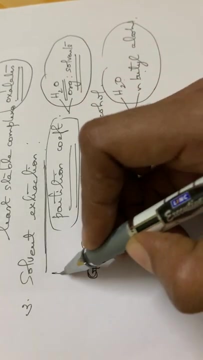 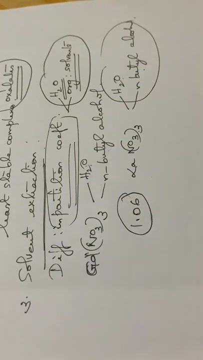 alcohol. Okay. The partition coefficient of gadolinium nitrate between water as well as in b Romeo3: thrice it is 1.06 times greater than that of lanthanum nitrate in water, as tanto between water as well as organic solvents. okay, so that is the point here. 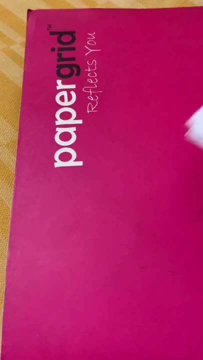 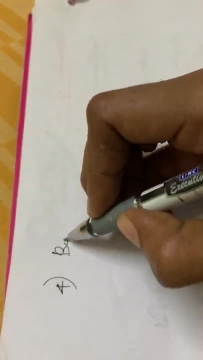 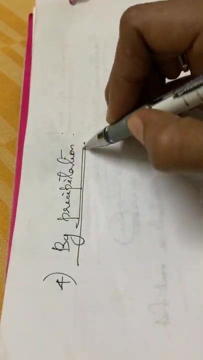 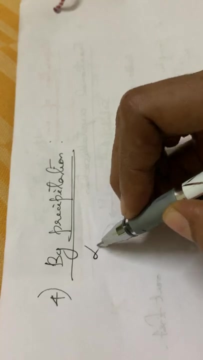 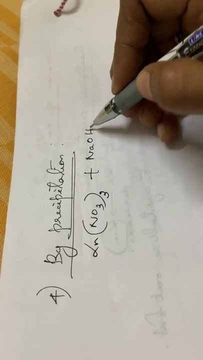 Then the next one, that is, by precipitation. the fourth one by precipitation. by precipitation, see, for example, when lanthanum nitrate, LNNO3 thrice, lanthanum nitrate, when treated with sodium hydroxide, sodium hydroxide and this here it is. here we have got a mixture of this. 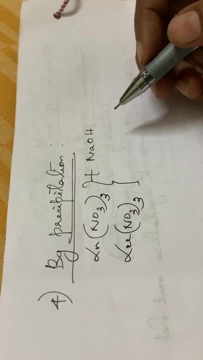 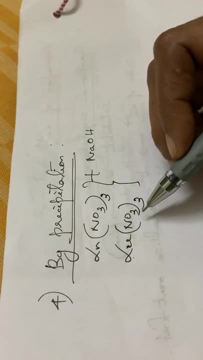 lanthanum nitrate as well as lutetium nitrate. when NaOH is added to this solution, to this mixture of these two, what happens is that this, which one is it is the weakest base- lanthanum or lutetium? Lutetium is the weakest base. 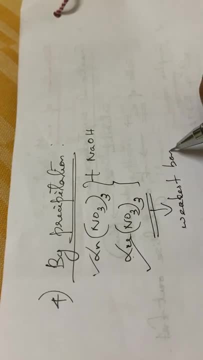 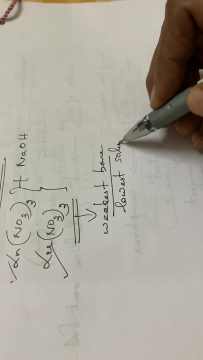 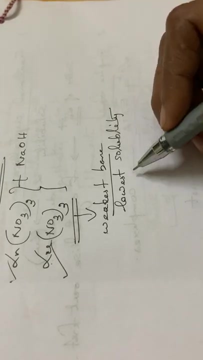 Lutetium is the weakest base. So weakest base means it has the lowest solubility. Weakest base means it is less soluble or it has the lowest solubility. and again, lowest solubility means which one will be a precipitating first. 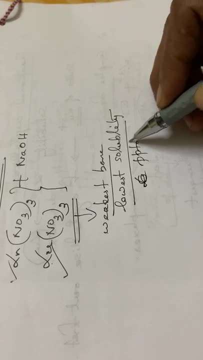 Lutetium will be precipitating first, precipitated first. So while taking a mixture of lanthanum nitrate and lutetium nitrate, Lutetium is the weakest base: Lutetium nitrate and lutetium nitrate in sodium hydroxide. 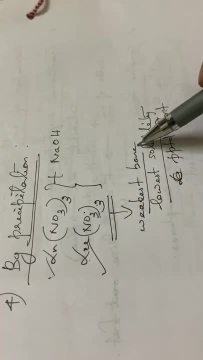 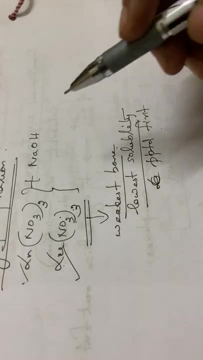 Since lutetium nitrate, it is the weakest base. we had already seen Weakest base and hence it has got the lowest solubility. so it will be precipitating first. But in the case of lanthanum nitrate it is a strongest base, isn't it? 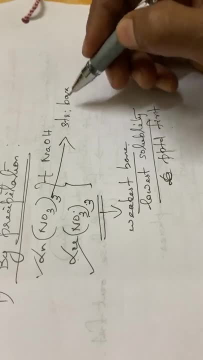 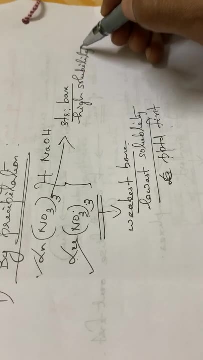 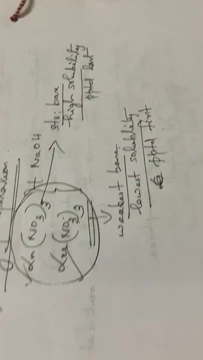 Just the reverse. lanthanum nitrate is the is a strong base, So what happens? It has got high, high solubility or highest solubility. So what happens? It will be precipitated last, Okay, Okay. So the mixture of lanthanum nitrate and lutetium nitrate treated with NaOH? this is the case. 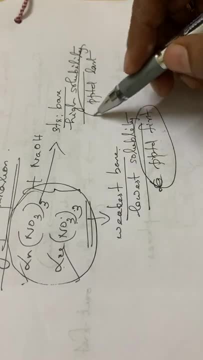 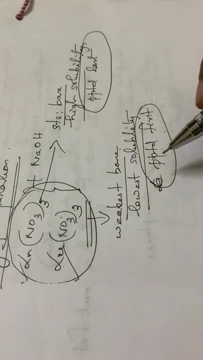 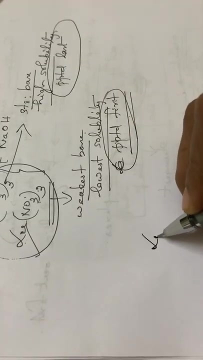 So lutetium nitrate will be precipitating out first and lanthanum nitrate will be precipitating out the last. Okay, So based on this, the lowest solubility substance will be precipitated out first. So here the principle used is the ion which has got the lowest solubility, the ion which 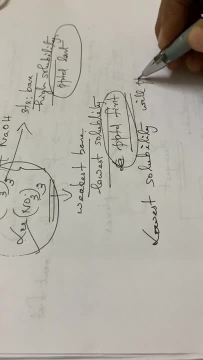 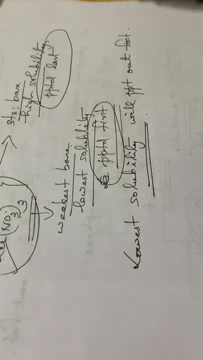 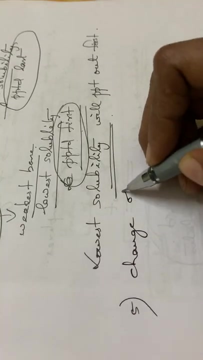 has got the lowest solubility will precipitate. Okay, So precipitate out first. That is the principle adopted here. Okay, So that is the fourth point. by precipitation, Then fifth one, by the change of oxidation state. By the change of oxidation state. 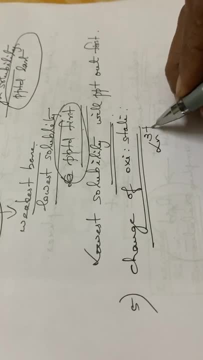 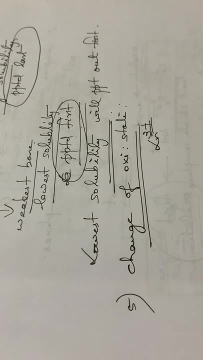 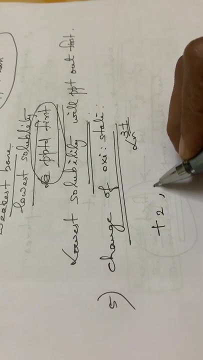 See, by changing the oxidation state generally we had seen this lanthanum. it is having a plus 3 oxidation state. Okay, See, for By changing this oxidation state We can separate these, Okay, These ions, very easily. Okay, That means sometimes an ion. it is having a plus 2 oxidation state, plus 4 oxidation state. 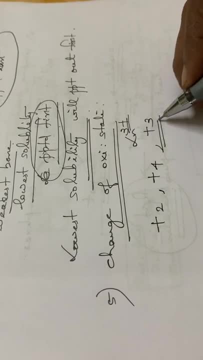 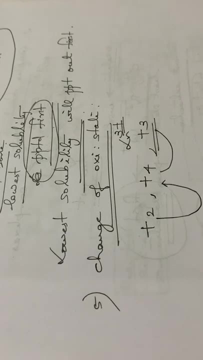 along with that, a plus 3 oxidation state will be there. Then we can separate the ion by changing the oxidation state, that is, from plus 2 we can change it to plus 4 or like that. Okay, So by changing the oxidation state of ions we can separate it easily. 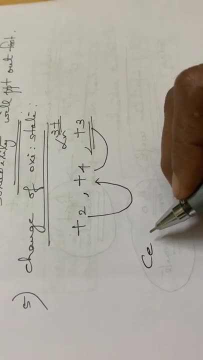 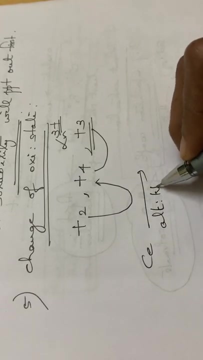 For example, from this lanthanid ion, lanthanum ions- the cerium can be treated with lutetium. Okay, Cerium can be treated with alkaline KMnO4.. See alkaline KMnO4. it is a very good oxidizing agent. 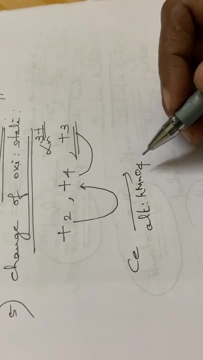 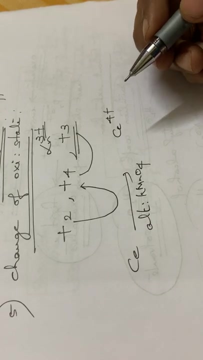 Okay, Cerium on treating with alkaline KMnO4. what happens is that this cerium, it is converted to cerium 4 plus, Its oxidation state changed to cerium 4 plus. See here in the solution. it may be in the form of cerium 3 plus. 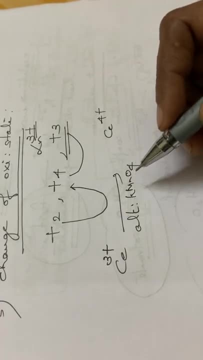 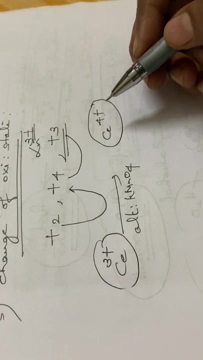 So we are converting it into cerium 4 plus by oxidizing using alkaline KMnO4.. See what about the charge. The charge is increased From cerium 3 plus to 4 plus. So what happens while the charge is increased? this? what about the size of the ion? 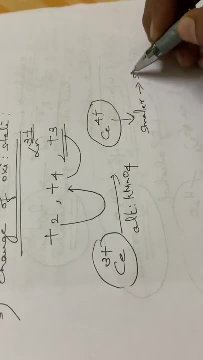 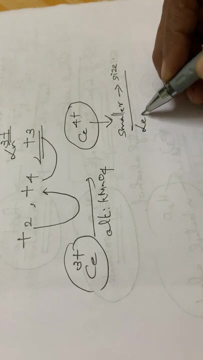 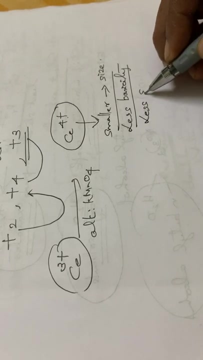 Size will be getting smaller, isn't it Smaller size while going through cerium 4 plus? So size smaller means that its basic nature will be less, isn't it? It has got a less basicity. Size smaller, so less basicity. then less basicity means it has got a less solubility while comparing. 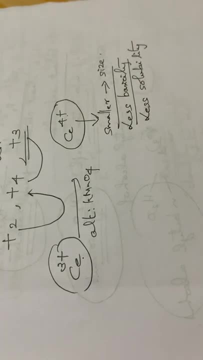 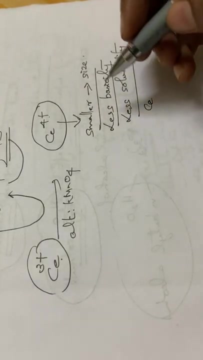 with that of cerium 4 plus. So less basicity and then less solubility. So this what happens? the cerium, it will be precipitating a cerium hydroxide. Cerium 4 plus means it can be cerium 4 times. 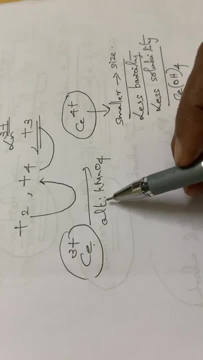 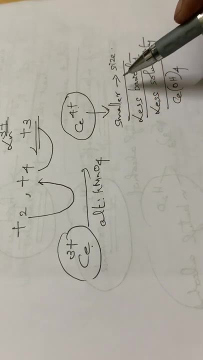 Okay, So by just by just the treatment, treating, using, sorry, by treating alkaline KMnO4, this 3 plus, it is oxidized to 4 plus and thereby the size is reduced. basicity becomes, became less, then solubility again goes less. 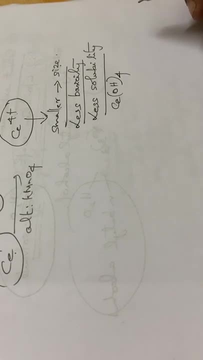 Then we will be oxidizing, Then we will be obtaining it as cerium hydroxide. okay, So the cerium hydroxide, it can be precipitated by treating with an alkali, isn't it? So by treating with an alkali, we will be having cerium hydroxide. 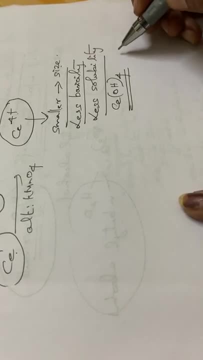 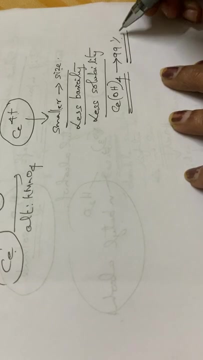 So by this method, we will be obtaining very, very high pure solution. okay, That means it is about this: obtained a cerium hydroxide. it is about 99 percentage pure. okay, This is another important point to be noted. okay, Okay, Thank you. 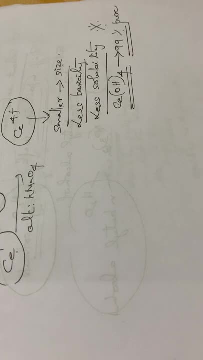 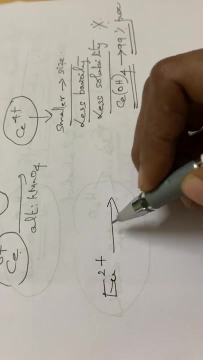 So this is regarding the oxidation state. Similarly, so many ions can be converted, that is, europium 2 plus Europium 2 plus. it can be reduced using zinc amalgam. Zinc amalgam, it is a very good reducing agent, isn't it? 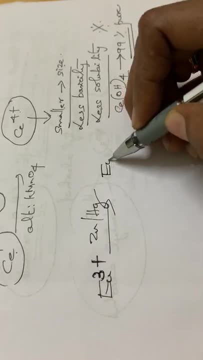 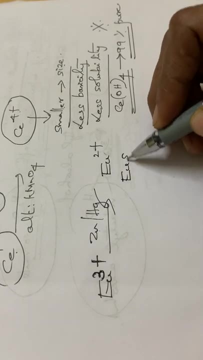 Sorry, europium 3 plus. it is reduced to europium 2 plus. Europium 3 plus. reduced using zinc amalgam, it is reduced to europium 2 plus. That means it can be in the form of sulfates, that is, europium sulfate. 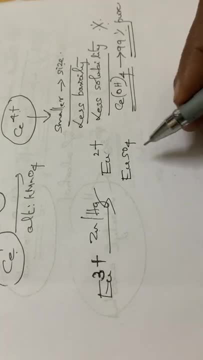 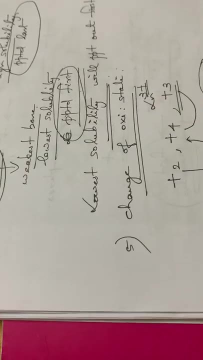 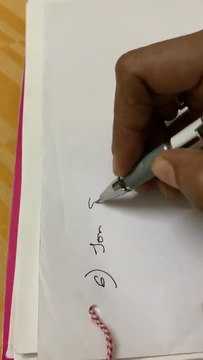 Okay, Okay, And then we can precipitate out this europium sulfate. So this is another method: change of oxidation state. And then the last method, that is, by ion exchange method. Sixth one: by ion exchange method. You have heard of ion exchange resins, isn't it? Here also ion exchange resins are used for the separation of lanthanides. okay, So here this ion exchange resin is used. Ion exchange resin is used. Ion exchange resin is used for the separation of lanthanides, and also usually this ion exchange resins, it will be having a functional group of either COOH or SO3H. 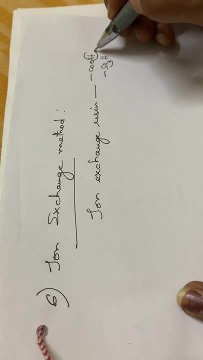 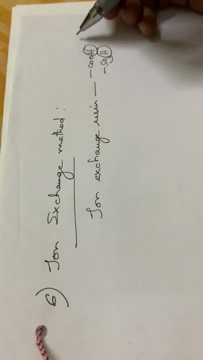 What is the peculiarity of these two groups? It has got an H plus, isn't it? An H plus will be removed easily. So this resin. it is packed in a column, See column means it is just a bigger size than that of a burette. 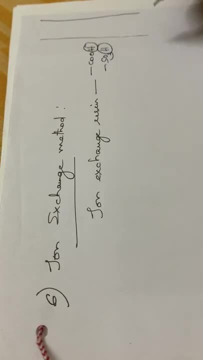 Okay, It is a long column. It will be like this: It will be very thicker one while comparing with that of burette, but almost the same pattern. okay, And also this is filled with the ion exchange resins. okay, This is called as a column and it is filled with the ion exchange resin. 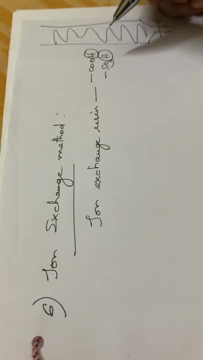 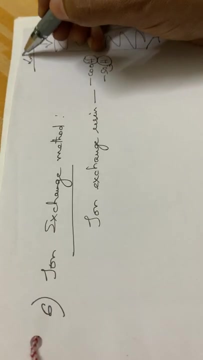 And usually this resin it has got a COOH or an SO3H group. that means an acetic group is filled in as a column. Then the mixture, the lanthanide mixture, to be separated. we are adding through this portion: okay, The solution to be separated. 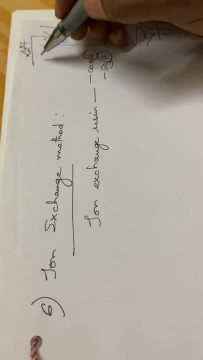 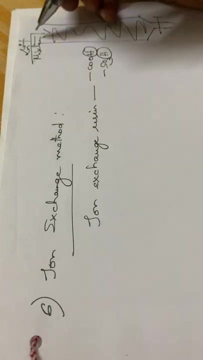 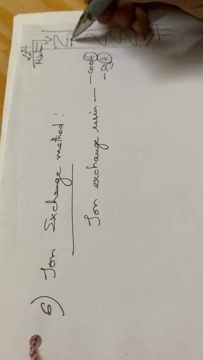 That means the lanthanide solution to be separated. Okay, The solution to be separated or the mixture to be separated. it is passed over through this solution And also this solution, it is allowed to run down through the column. So what happens is that this lanthanide ions- see here, if we are taking a COOH group resin. 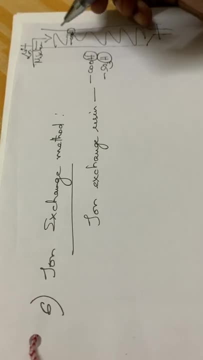 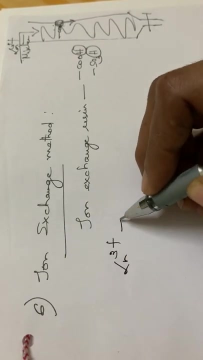 here. what happens is that this H plus will be replaced by the coming lanthanum ions. Okay, This H plus ions will be will be removed and in that position, this lanthanum ions will take that position. okay, So we can write the equation that is lanthanum 3 plus. it will be reacting with the hydrogen. 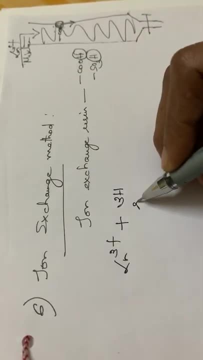 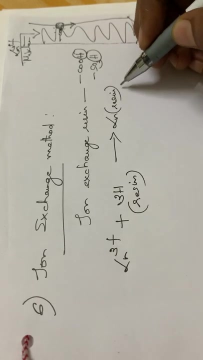 present H plus ion present in the resin or the hydrogen ion present in the resin. So what happens? we will be having the lanthanide ions. it will be attached to the resin, that is ln resin. thrice will be forming and the H plus will be removed and the H plus will. 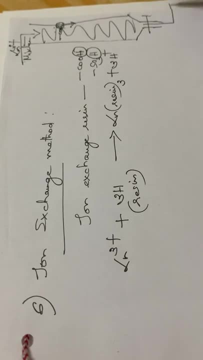 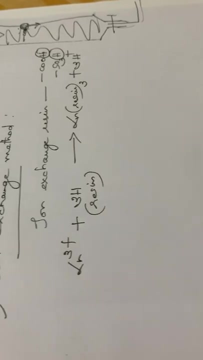 be going through here. Okay, And this: we can remove the H plus ions or the H plus ions, Okay. Okay, So we have removed the ionic solution from from the bottom. Okay, Then you have to add a buffered solution of citric acid. 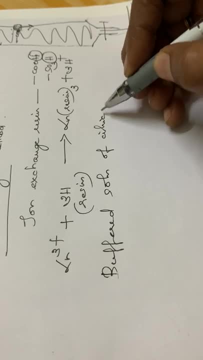 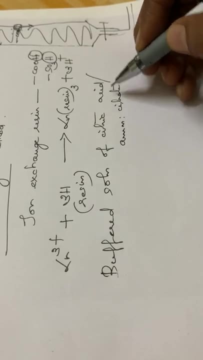 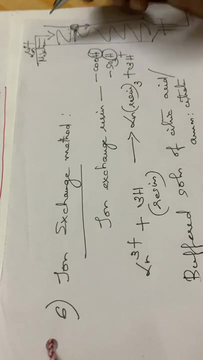 We have to add a buffered solution of citric acid, buffered solution of citric acid or ammonium citrate. So from the top of the column we have to add a buffered solution of citric acid or ammonium citrate. So this solution. 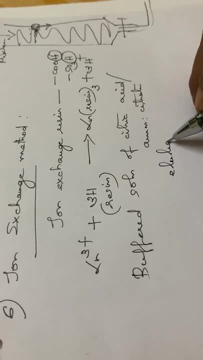 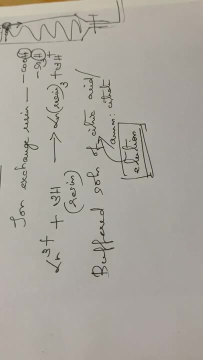 It is used for elution, the process it is called as elution. Okay, So for elution we are using this particular solution, citric acid or ammonium citrate solution. So here, as the citrate solution runs down, what happens is that the lanthanum ions the 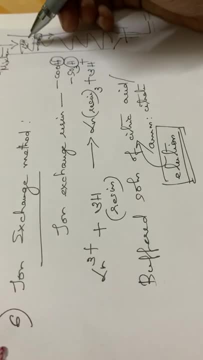 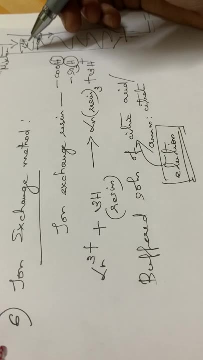 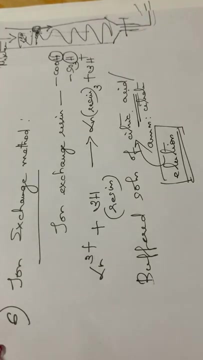 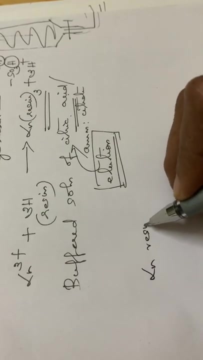 ln 3 plus. it will be attaching in the in this column, in this resin, isn't it? So this ln 3 plus ions it will be. it will be forming complexes with the citrate. Okay, So this already here. it is present in the column in lanthanum resin thrice it will be. 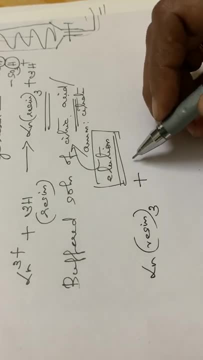 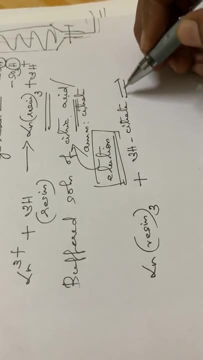 there isn't it in the column, it will be there. So to that we are adding the citrate solution 3H, then citrate- it is a citric acid solution, citrate. then what happens is that we will be having 3 hydrogen and it will be remaining. 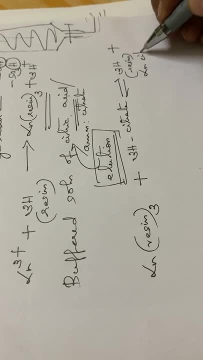 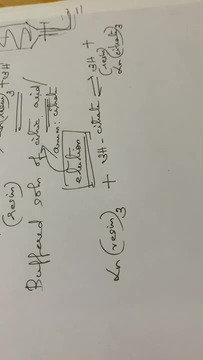 in the resin plus lanthanum citrate, That is, a lanthanum citrate solution. Okay, So the citrate complex is a complex will be formed and it will be coming out through this, through this portion. Okay So this citrate complex comes down. what happens? the lanthanum 3 plus also will be coming along. 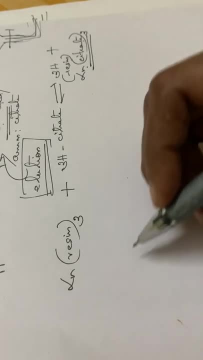 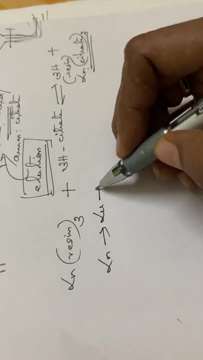 with the citrate ion, Okay, And also see the lanthanate ions. from lanthanum to lutetium, the ionic size is varying, isn't it? Lutetium, it is having a smaller size. Lutetium, it is having a smaller size. 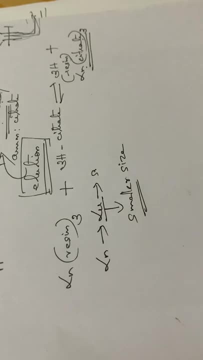 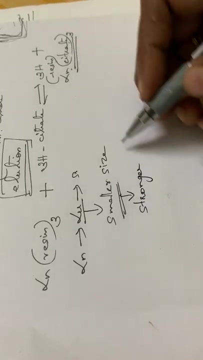 Okay, Smaller size and also, since this smaller size ion, it can form stronger complexes, isn't it? The complex formed will be a stronger, that is, the lanthanum citrate or the lutetium citrate complex will be a stronger one, isn't it? 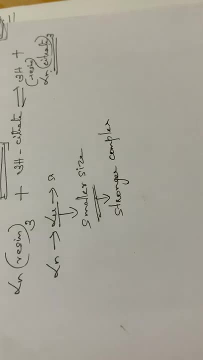 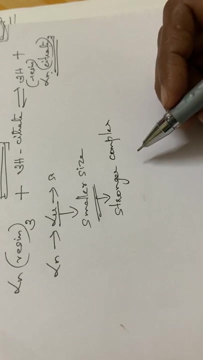 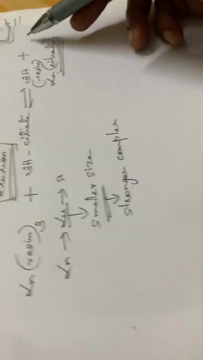 Stronger complex can be formed. a stronger complex can be formed, isn't it? And again, what happens is that the smaller and the smaller complex and the heavier ion, So which ion will be coming first from this, so from this portion lanthanum, lanthanum citrate. 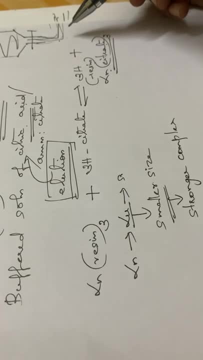 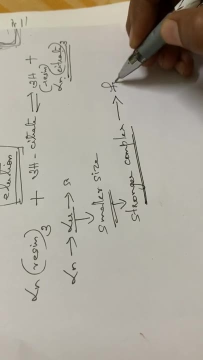 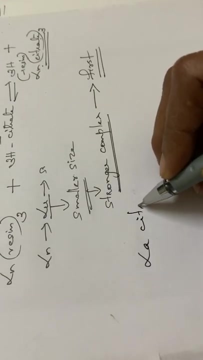 or the or lutetium citrate. Lutetium citrate will be coming out first. Okay. Stronger complex means this: lutetium citrate complex will comes out first from the, from the column Okay, Then the last come will be the lanthanum citrate complex. 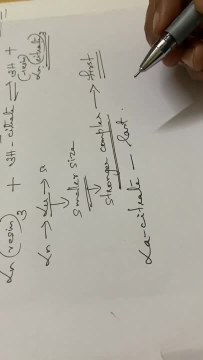 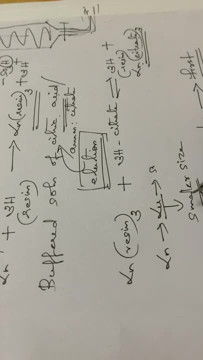 Lanthanum citrate complex comes out last. Okay, So smaller and the heavier ions will be eluted first. Okay, Smaller and the heavier ions will be eluted first. That means lutetium nitrate complex will be coming out first. 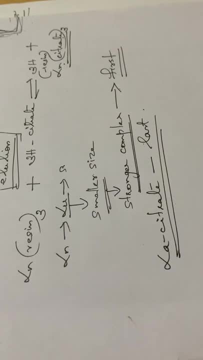 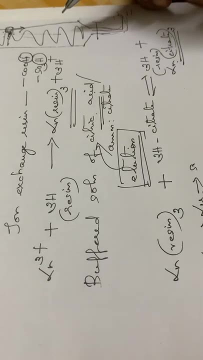 Then, in the last stage, only this lanthanum citrate complex will be coming out. Okay, So this is the. so in this way we can separate similarly. so after lutetium, then comes the next ion, next ion, citrate complex. So in this way we can separate all the ions from this. 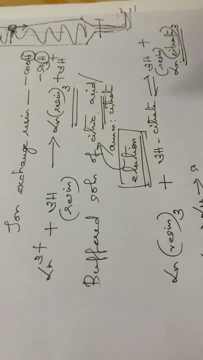 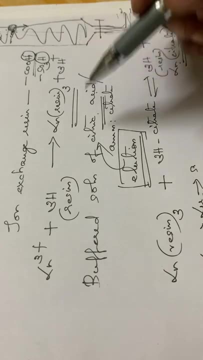 Okay, So this is the ion exchange resin. So in ion exchange resin we are using an COH group or an SO3H group resin. Then it is lanthanate solution. it is passed over the resin, So it will be forming a complex. 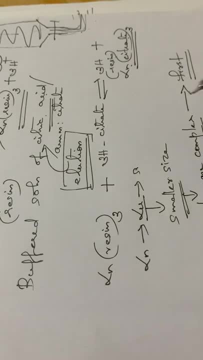 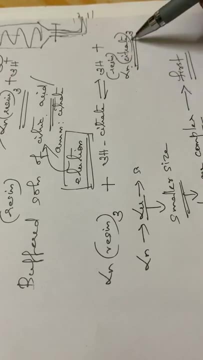 Then we are adding buffered solution of citric acid or ammonium citrate as an elution, as an eluting agent. So then, this lanthanum resin, it will be combining with the citrate to form a complex, that is, the lanthanum citrate complex. 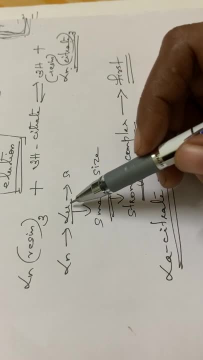 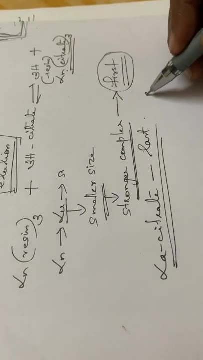 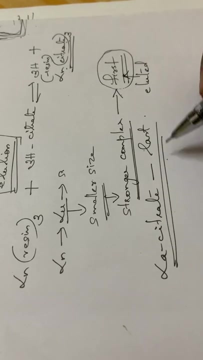 So, starting from lanthanum to lutetium, the ionic size decreases. Lutetium is the smallest ion, and hence it forms a stronger complex, and then it will be eluted. first It is eluted. Okay, The process in this citrate is sorry. lutetium citrate is eluted first and lanthanum citrate. 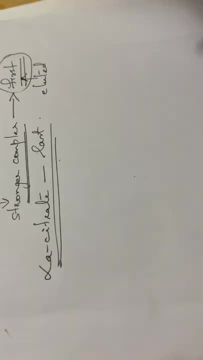 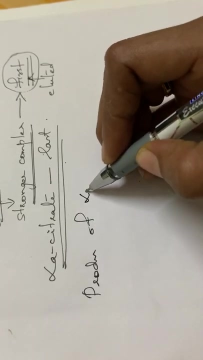 is eluted last. Okay, Then the next is this: production of lanthanate metals. Some of the another title you have to study is the production of lanthanate metals. that is, the different methods for the production of lanthanate metals. Okay, 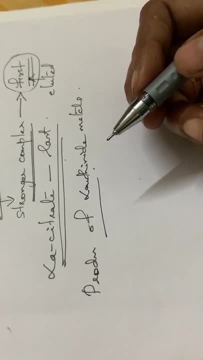 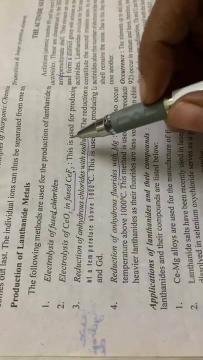 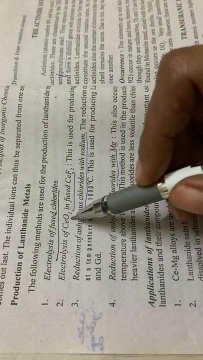 So lanthanate metals. I think you can read from the, from the textbook. I will go through this also. See lanthanate metals. see here the first one, that is, the following: methods are used for the production of lanthanates: first one: electrolysis of fused chlorides. second one: electrolysis 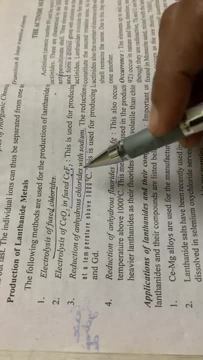 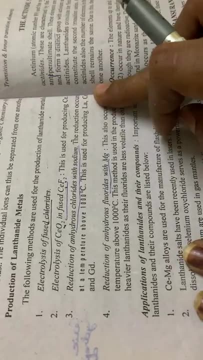 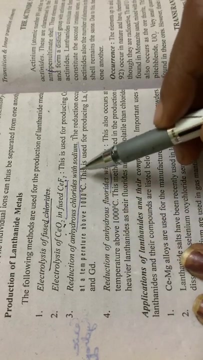 of CeO2 infused. CeF2, that is, cerium oxide, is electrolysis of CeO2. it is electrolyzed. This is used for producing cerium. Okay, Cerium oxide. in the presence of CeF2, cerium fluoride. Then the third one: reduction of anhydrous chlorides with sodium. 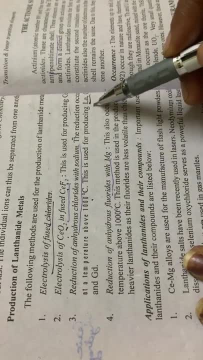 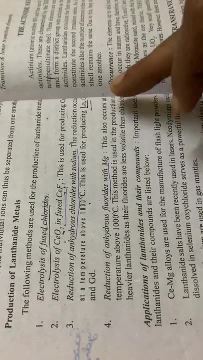 The reduction occurs at a temperature above 1000 degree. This is used for producing lanthanum, then cerium and gadolinium. Okay, The temperature above 1000 degree we are reducing. Okay. Then reduction of anhydrous fluorides with magnesium. 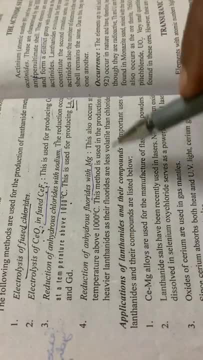 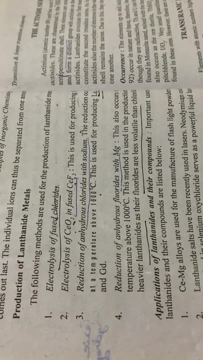 Here we are using a temperature of 1000 degree. This is also used in the production of heavier lanthanates. Okay, So These are the methods of production of lanthanate metals that you have to read all the all this sometimes may be asked in any part: two marks or four marks. 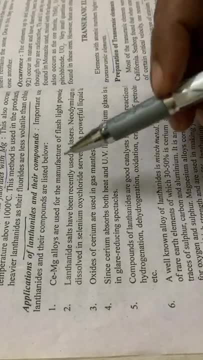 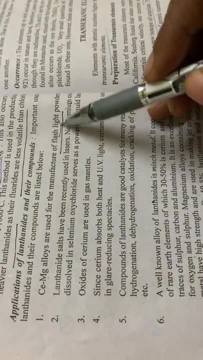 Okay, Then the next is the application of lanthanates and their compounds. See here lanthanates and their compound. some of the uses are there. that is cerium magnesium alloys- it is used in the manufacture of flashlight powders. Then lanthanate salts: it is used in lasers. neodymium oxide: it is dissolved in selenium. 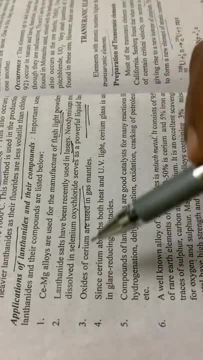 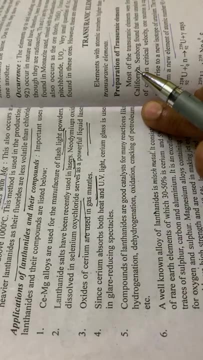 oxychloride used as a powerful liquid laser- Okay. Then oxides of cerium used in gas manufacturing- Okay. It is used in glass mantles, then cerium. it is absorbing heat and UV light and, as a result, cerium glass- it is used in glare, reducing spectacles. 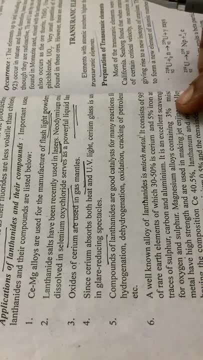 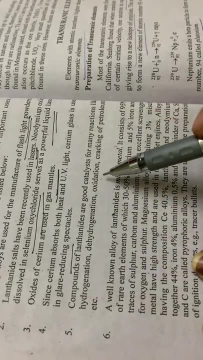 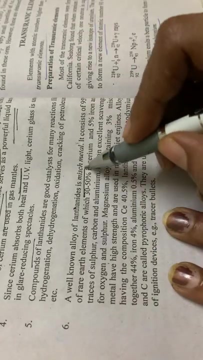 So cerium. it is used in glare reducing spectacles. this uses or applications it is very important. Then, compounds of lanthanates are good catalysts for many reactions like hydrogenation, dehydrogenation, oxidation, cracking of petroleum, etc. Then the last one, lanthanates. it is a well known alloy. it is mesh metal. 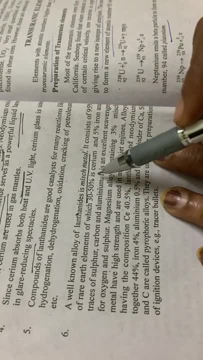 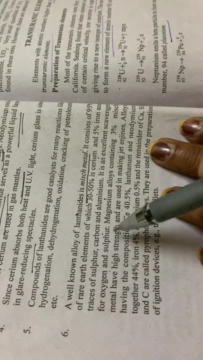 Okay, That means it consists of 30 to 35, 50 percentage of cerium, 5 percentage of iron, then traces of sulphur, carbon and aluminium. it is an excellent scavenger for oxygen and sulphur. magnesium alloys containing 3 percentage mesh metal have high strength and are used in making. 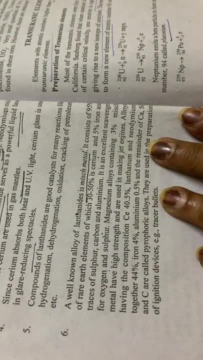 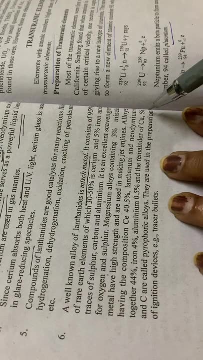 jet engines. alloys having the composition cerium 40.5 percentage, lanthanum and neodymium together 44 percentage, iron 4 percentage, aluminium 0.5 percentage and the remainder of calcium, silicon and carbon are called as pyrophoric alloys. Okay, 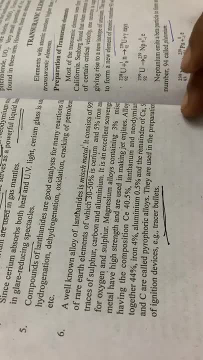 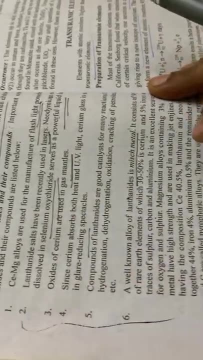 They are used in the preparation of ignition devices, example, tracer bullets. So these are some of the uses. you have to go through all these uses. just read all these things, okay? So this is regarding the application of lanthanates uses. it may be asked to sometimes, so please. 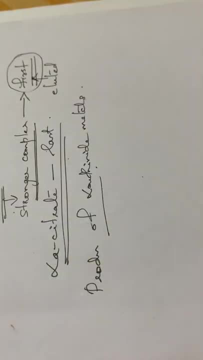 go through it and the next series, that is the actinide series that we can see in our next session. Thank you, 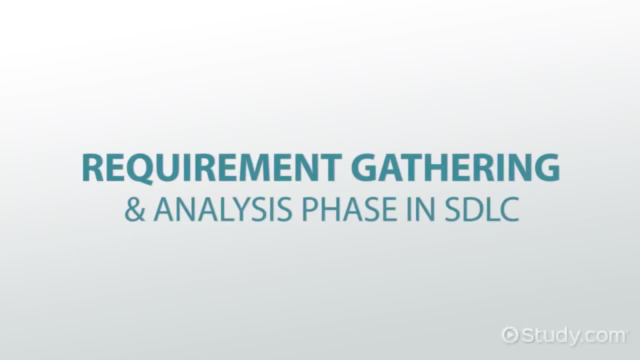 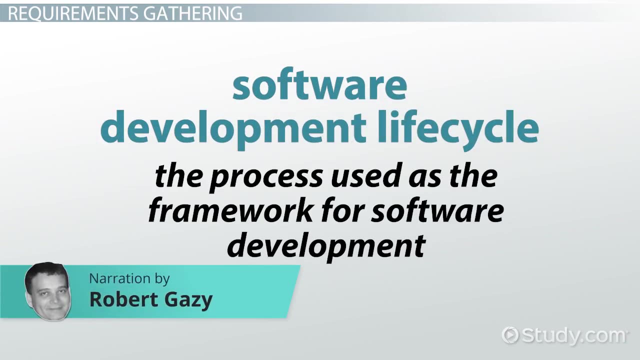 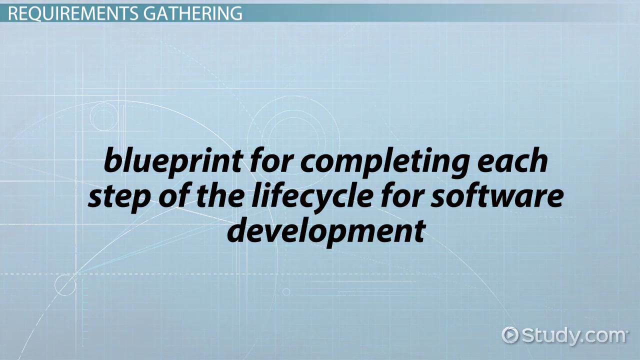 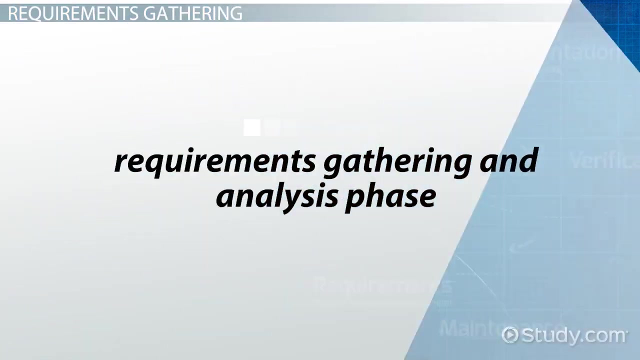 SDLC is an acronym for Software Development Lifecycle and is the process used as the framework for software development. Project managers and business organizations use the SDLC as a blueprint for completing each step of the lifecycle for software development. Each step of the SDLC is called a phase. The Requirements Gathering and Analysis phase is the first. 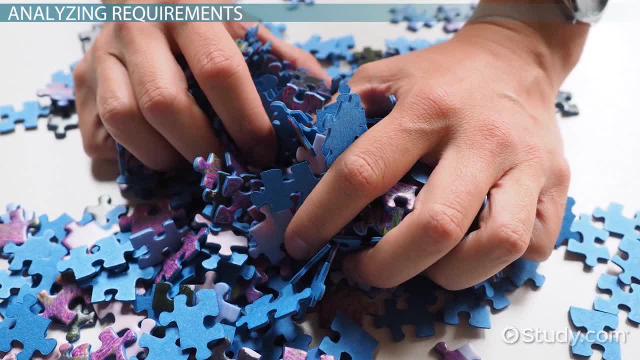 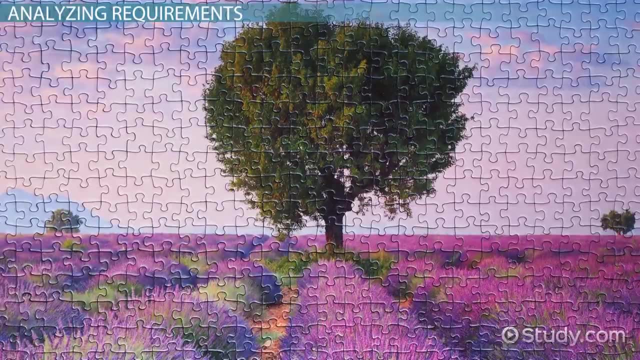 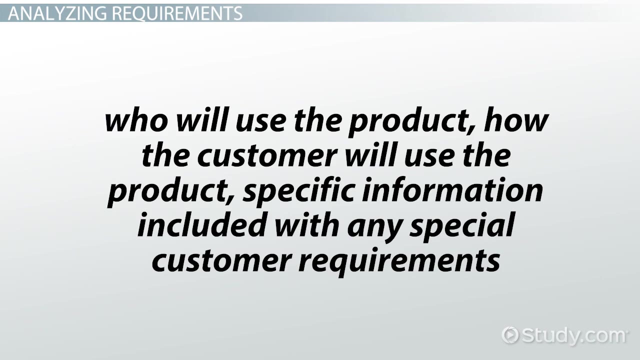 phase of the SDLC- Gathering requirements for the project is the most important part of the SDLC for project managers and internal stakeholders of a project. During this phase, the customer states the expectations of the project, including who will use the product, how the customer will use the product and the specific information included with any 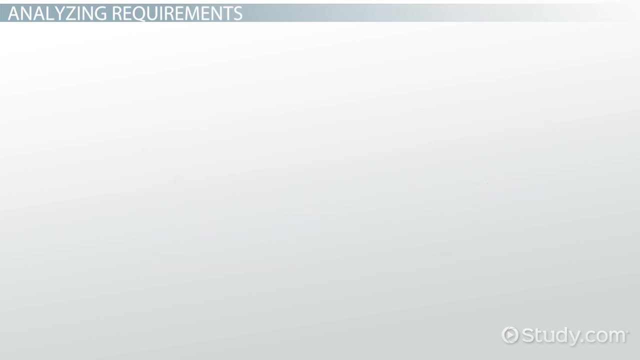 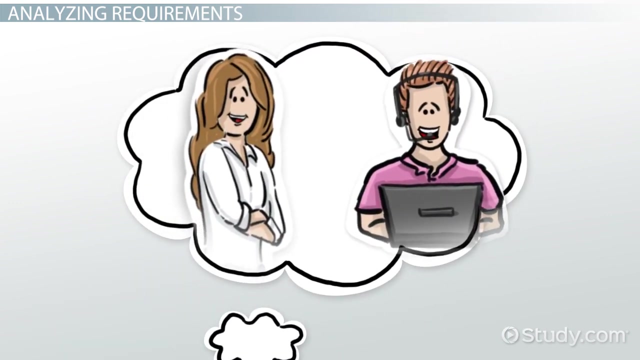 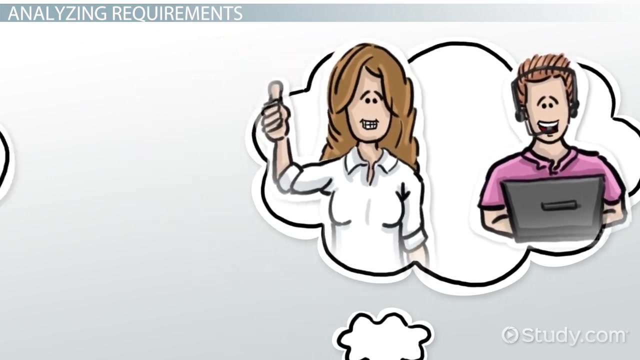 special customer requirements related to the software. The customer meets with business managers and analysts to provide the requirements. It's important for the project to be a project team to understand the needs of the customer because this information is critical to developing the product the customer requests After the customer provides requirements for.